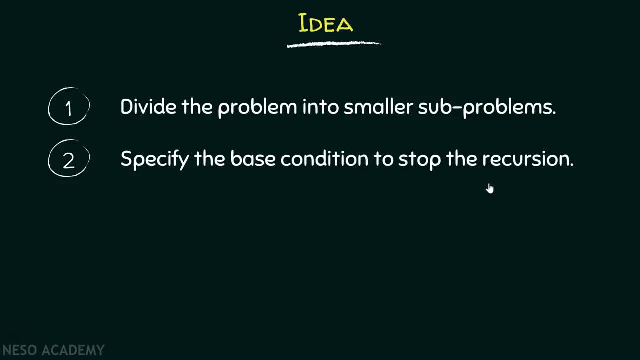 then it may go into infinite loop. It is very important to specify the base condition in your program. With the help of these two steps, we can write our recursive program very easily. Now let's see, with the help of a problem that, how we can implement these two steps. 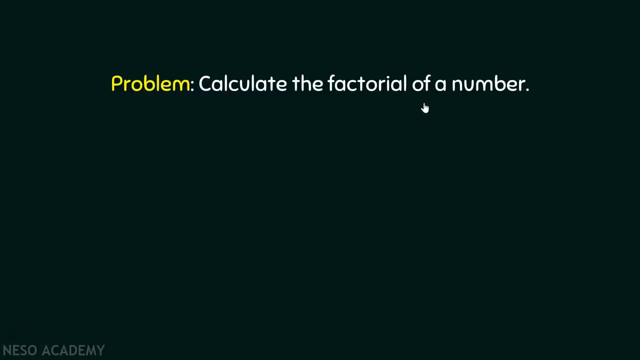 Our problem is calculate the factorial of a number. Now, what is factorial of a number? Suppose we want to calculate factorial of five, Then factorial of five is equal to five into four, into three, into two, into one Right, Which is equal to one twenty. 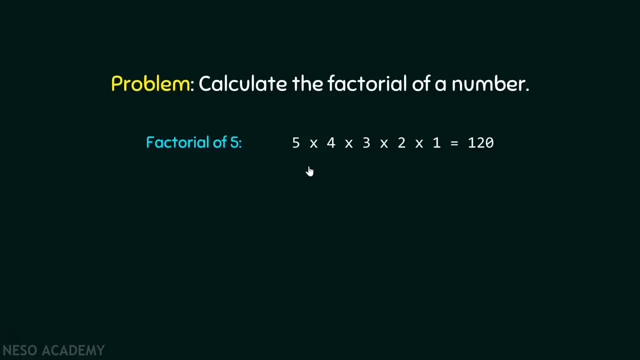 If we want to calculate factorial of six, then it will be six into five, into four, into three, into two, into one, which is simple to calculate. In order to write a recursive procedure for factorial of any number, you first have to specify what is going to be. 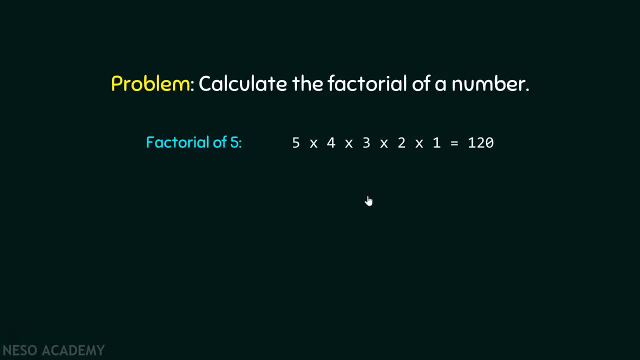 the basic structure of that program. Let's see what will be the basic structure. This is how basic structure of any recursive program looks like. It consists of one if construct and one else construct. If construct is the place where you will specify your base case. 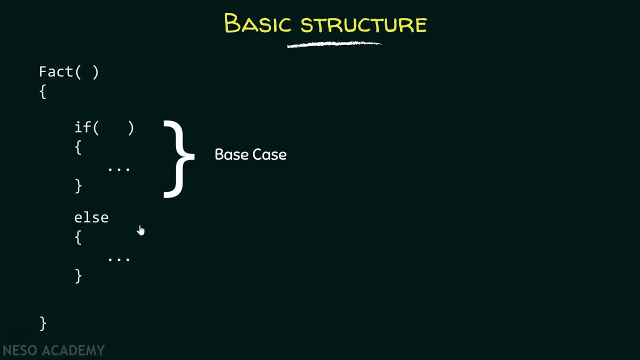 Please remember this point, And else construct is the place where you will specify your recursive procedure. In order to write any recursive program, the first thing you must specify is recursive procedure. Then you progress to your base case. Recursive procedure is the first thing. 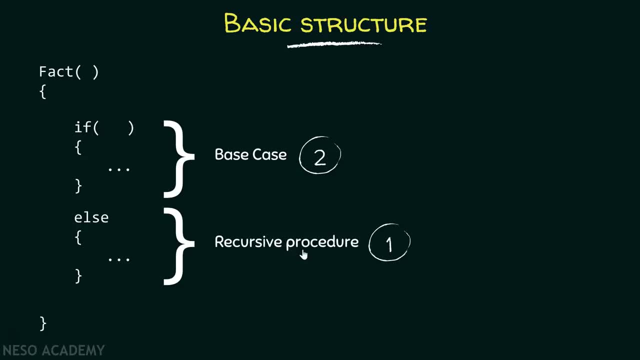 you must write down, Because this is very important to write. After that, specifying the base case will be cakewalk for you. Okay, Now, after understanding this basic structure, let's try to implement our steps, which we have already seen. First step is divide the problem. 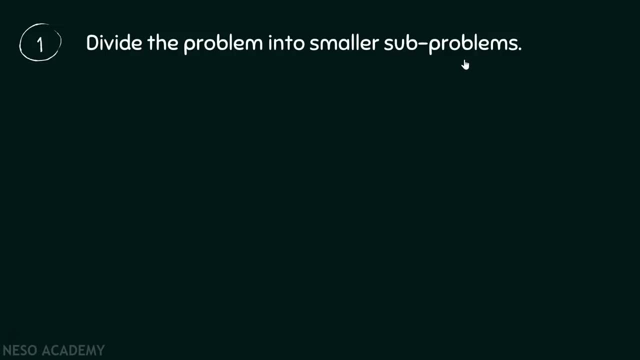 into smaller sub-problems. You have one problem, as in our case, is factorial. We need to divide our problem into smaller sub-problems so that we can actually attack the problem very easily. Suppose we want to calculate fact of four, which means factorial of four. 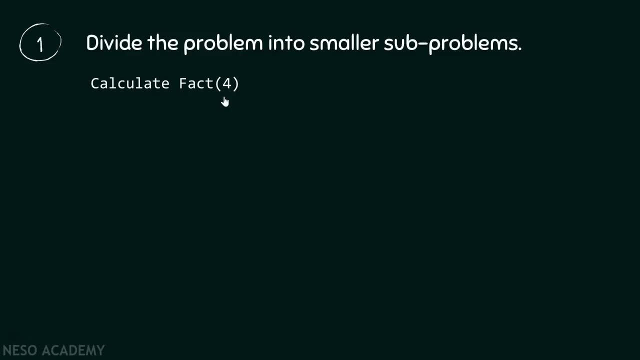 Now how we can divide this problem into smaller sub-problems. Think of a problem which is very easy to solve Like: suppose fact of one, Fact of one is equals to one. There is nothing you have to do explicitly in order to calculate factorial of one. 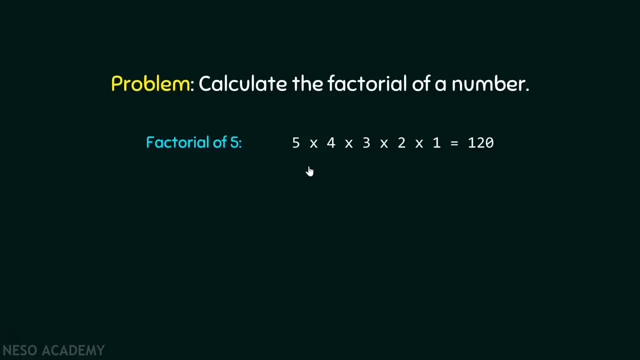 If we want to calculate factorial of six, then it will be six into five, into four, into three, into two, into one, which is simple to calculate. In order to write a recursive procedure for factorial of any number, you first have to specify what is going to be. 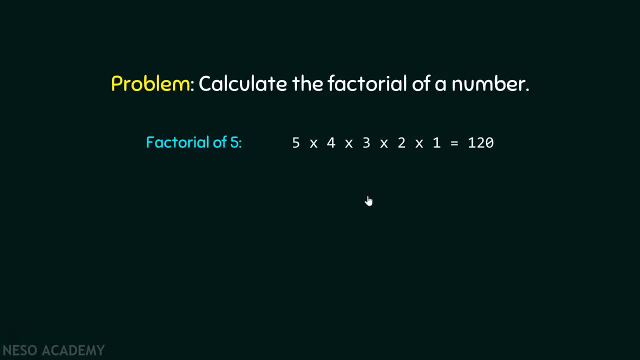 the basic structure of that program. Let's see what will be the basic structure. This is how basic structure of any recursive program looks like. It consists of one if construct and one else construct. If construct is the place where you will specify your base case. 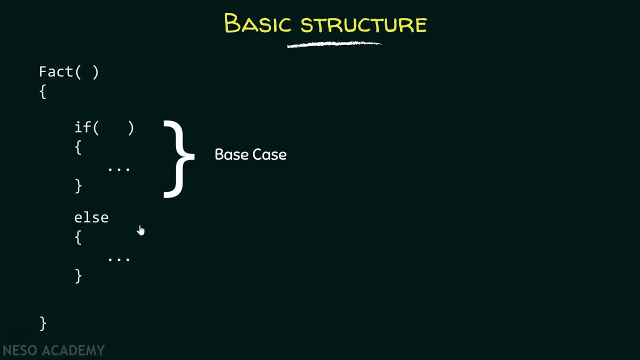 Please remember this point, And else construct is the place where you will specify your recursive procedure. In order to write any recursive program, the first thing you must specify is recursive procedure. Then you progress to your base case. Recursive procedure is the first thing. 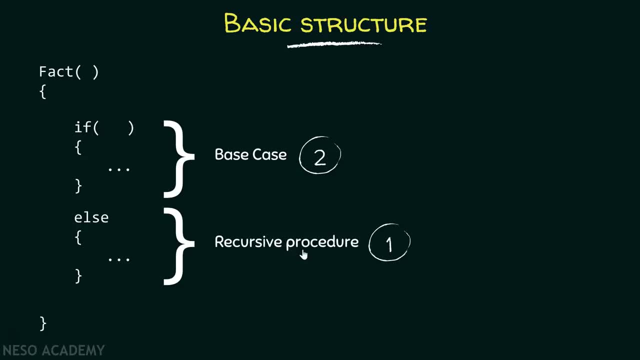 you must write down, Because this is very important to write. After that, specifying the base case will be cakewalk for you. Okay, Now, after understanding this basic structure, let's try to implement our steps, which we have already seen. First step is divide the problem. 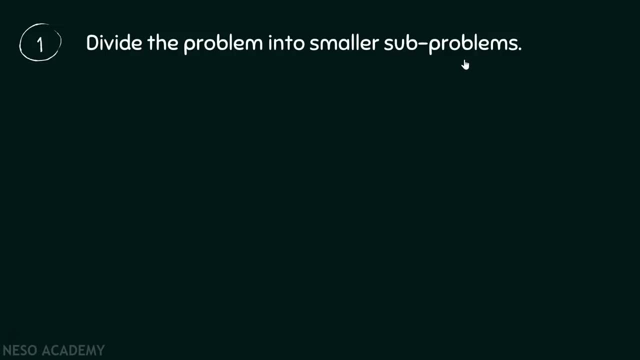 into smaller sub-problems. You have one problem, as in our case, is factorial. We need to divide our problem into smaller sub-problems so that we can actually attack the problem very easily. Suppose we want to calculate fact of four, which means factorial of four. 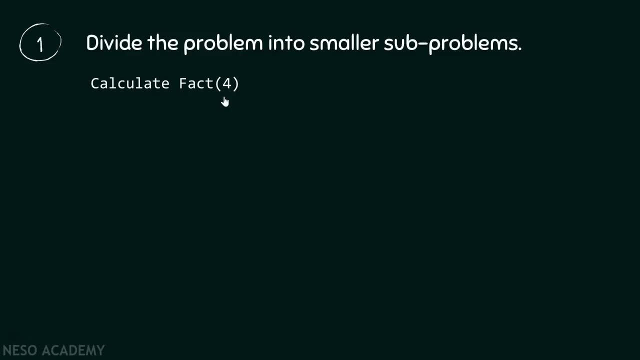 Now how we can divide this problem into smaller sub-problems. Think of a problem which is very easy to solve Like: suppose fact of one, Fact of one is equals to one. There is nothing you have to do explicitly in order to calculate factorial of one. 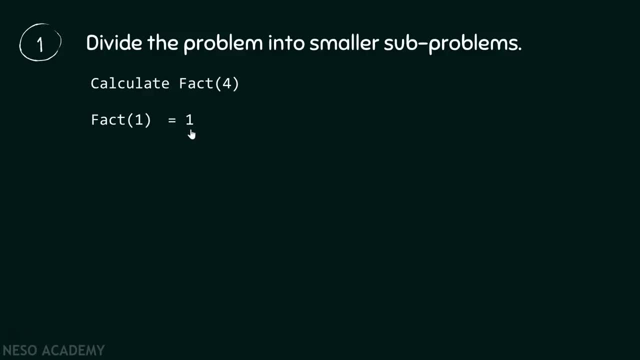 Factorial of one is equals to one. Now ask yourself this question: what is factorial of two? Factorial of two is equals to two into one, right, You already know this? Now, if you observe this very carefully, then we can replace this one by fact of one. 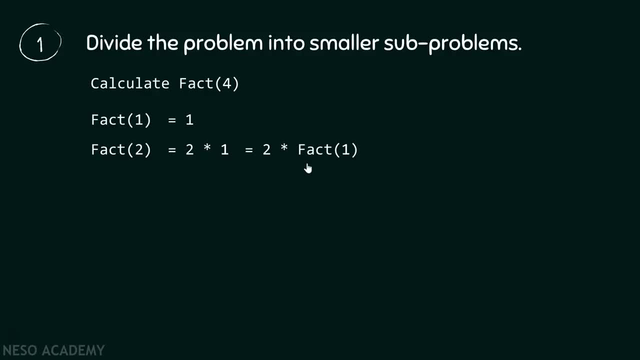 So we can replace this with two into fact of one. Both are one and the same, isn't that? so Now again ask yourself this question: what is fact of three? Fact of three is equals to three into two, into one right. 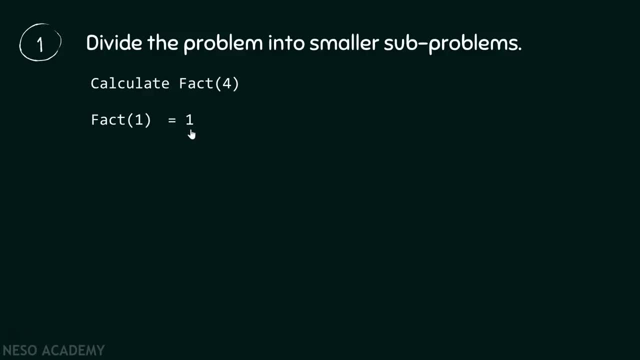 Factorial of one is equals to one. Now ask yourself this question: what is factorial of two? Factorial of two is equals to two into one, right, You already know this? Now, if you observe this very carefully, then we can replace this one by fact of one. 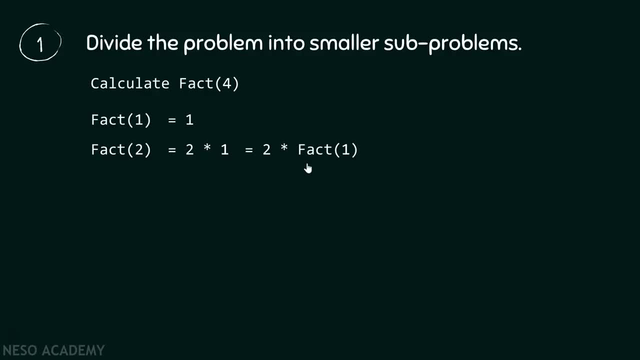 So we can replace this with two into fact of one. Both are one and the same, isn't that? so Now again ask yourself this question: what is fact of three? Fact of three is equals to three into two, into one right. 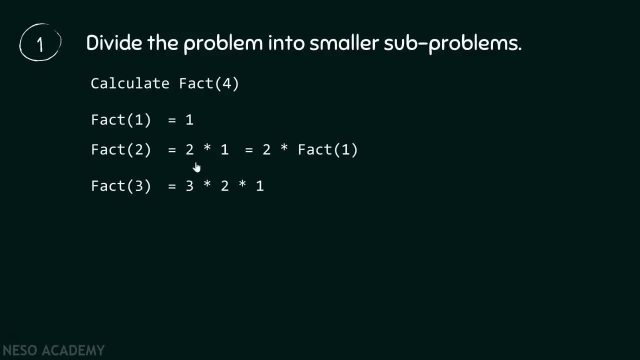 Now again, if you observe carefully, then you can write two into one as fact of two. So let me replace this with fact of two. This statement is equal to three into fact of two. This is how you will progress. Fact of four is equal to four into three, into two, into one. 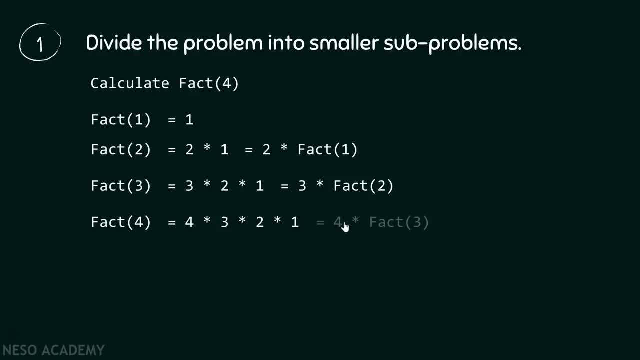 We can replace this whole statement by fact of three, right? So fact of four is equals to four into fact of three, And we have already calculated fact of three. You can clearly see how we are dividing our problem into smaller sub-problems. 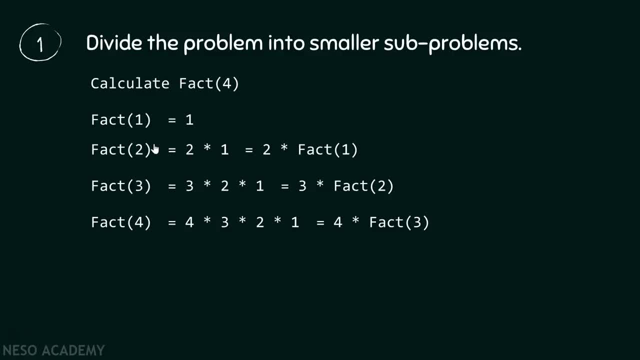 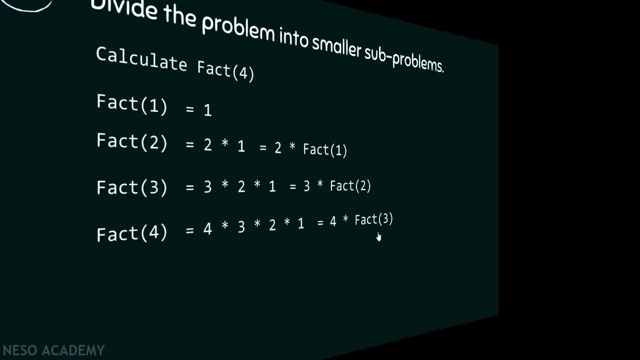 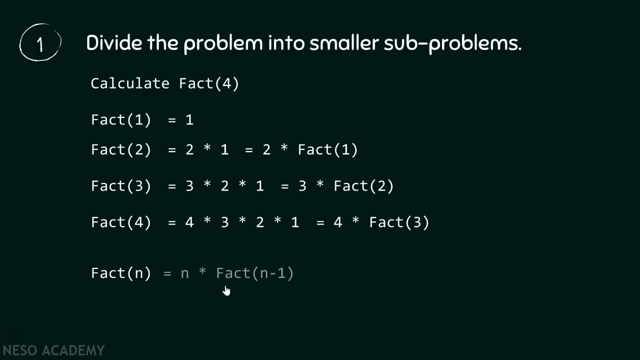 We started with the simplest possible solution and we progress gradually And then finally we end up with our solution, which is four into fact of three. Now if we want to calculate fact of n, then it is not very difficult to understand. Fact of n is equals to n into fact of n minus one. 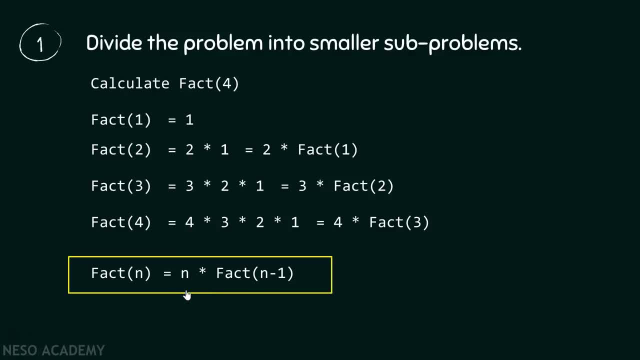 This is our recursive procedure because in general we have to write variable n right. Your program should not work according to n equals to four. it should work in general, right. That is why I am specifying fact of n And fact of n is equals to n into fact of n minus one. 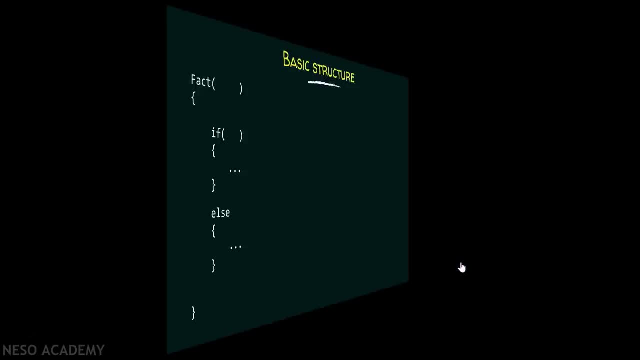 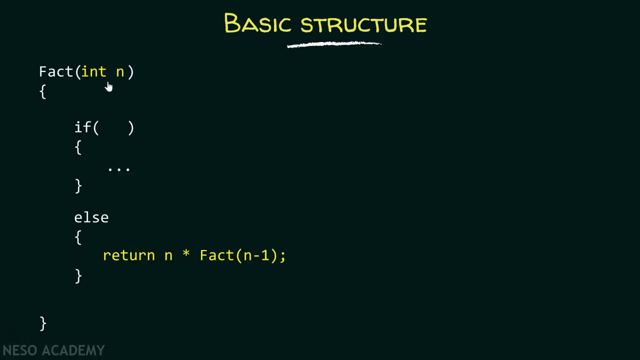 Simple. So what we can write in our else construct, We can simply write: return n into fact of n minus one- And here we should specify integer n, right, Because this is our variable n. and inside this else construct you simply write return n into fact of n minus one. 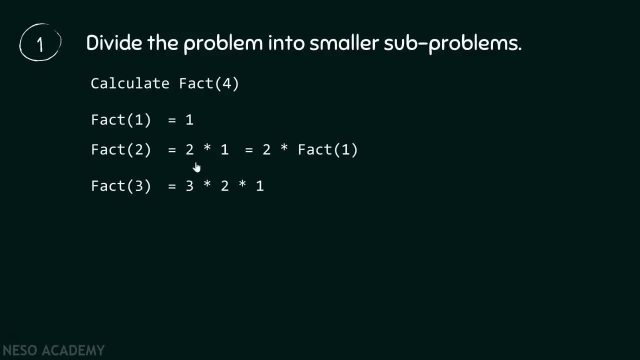 Now again, if you observe carefully, then you can write two into one as fact of two. So let me replace this with fact of two. This statement is equal to three into fact of two. This is how you will progress. Fact of four is equal to four into three, into two, into one. 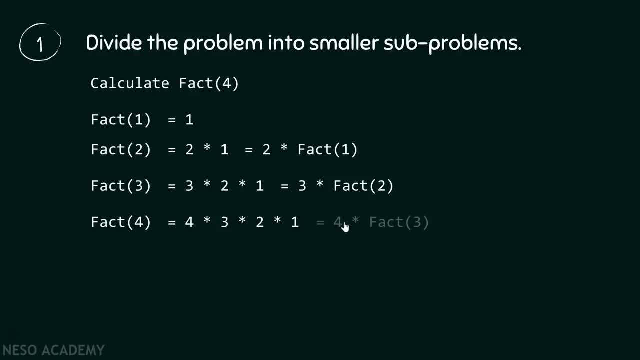 We can replace this whole statement by fact of three, right? So fact of four is equals to four into fact of three, And we have already calculated fact of three. You can clearly see how we are dividing our problem into smaller sub-problems. 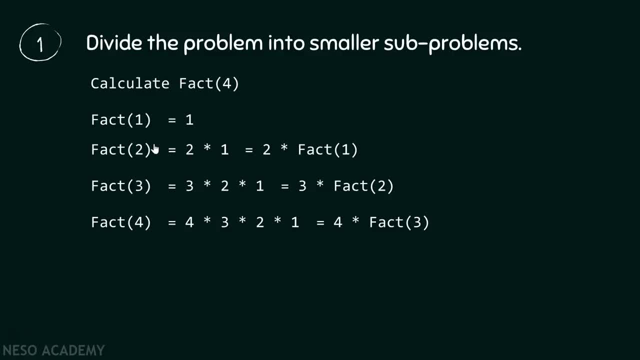 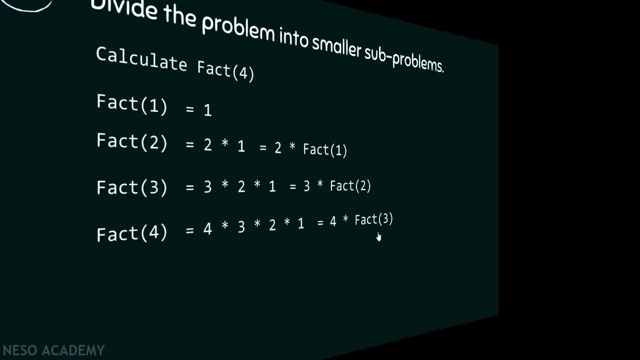 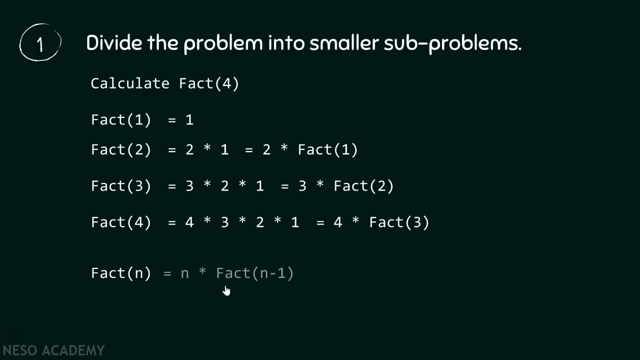 We started with the simplest possible solution and we progress gradually And then finally we end up with our solution, which is four into fact of three. Now if we want to calculate fact of n, then it is not very difficult to understand. Fact of n is equals to n into fact of n minus one. 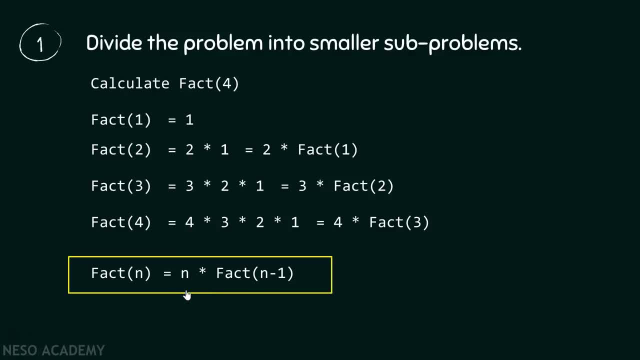 This is our recursive procedure because in general we have to write variable n right. Your program should not work according to n equals to four. it should work in general, right. That is why I am specifying fact of n And fact of n is equals to n into fact of n minus one. 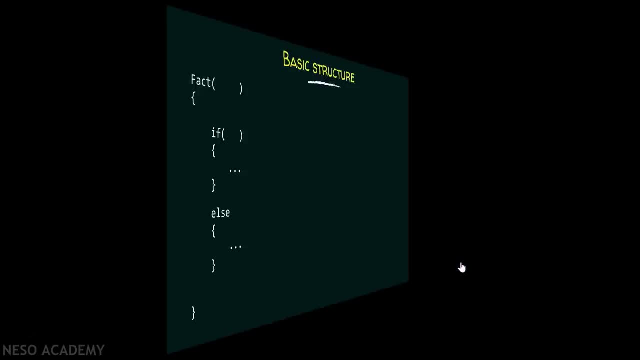 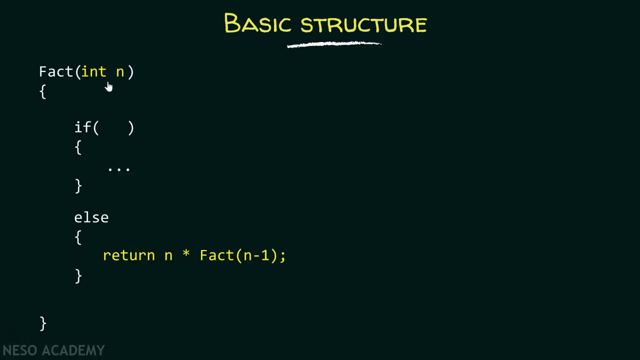 Simple. So what we can write in our else construct, We can simply write: return n into fact of n minus one- And here we should specify integer n, right, Because this is our variable n. and inside this else construct you simply write return n into fact of n minus one. 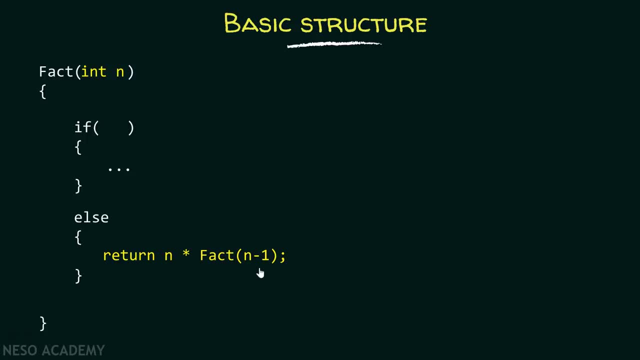 This is our recursive procedure. After completion of this recursive procedure, there is nothing much left in your code. You just have to specify the base condition, which is very simple to write. Now, for the sake of completeness, let's consider our second step. 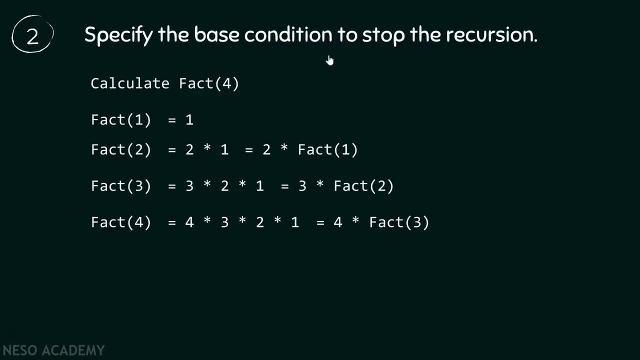 Second step is to specify the base condition in order to stop the recursion. Now, what is the base condition? What exactly is our base condition and what is the criteria of choosing the base condition? Base condition is the one which doesn't require you to call the same function again. 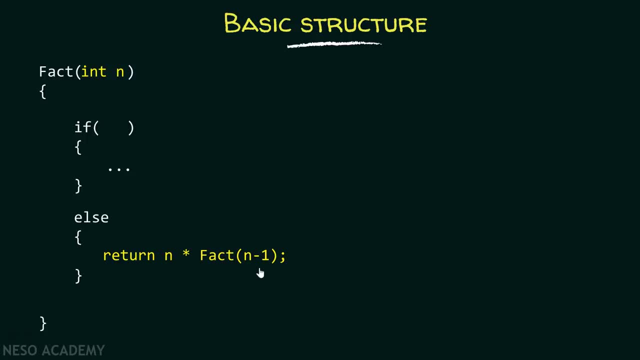 This is our recursive procedure. After completion of this recursive procedure, there is nothing much left in your code. You just have to specify the base condition, which is very simple to write. Now, for the sake of completeness, let's consider our second step. 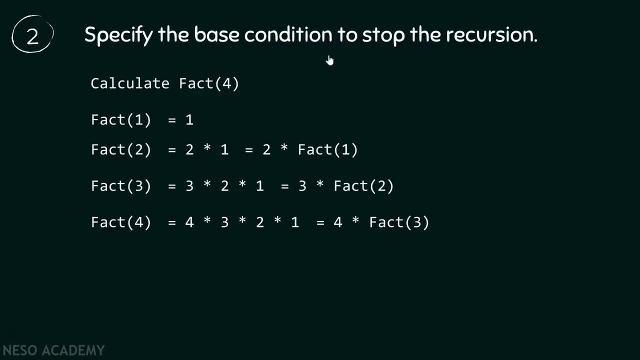 Second step is to specify the base condition in order to stop the recursion. Now, what is the base condition? What exactly is our base condition and what is the criteria of choosing the base condition? Base condition is the one which doesn't require you to call the same function again. 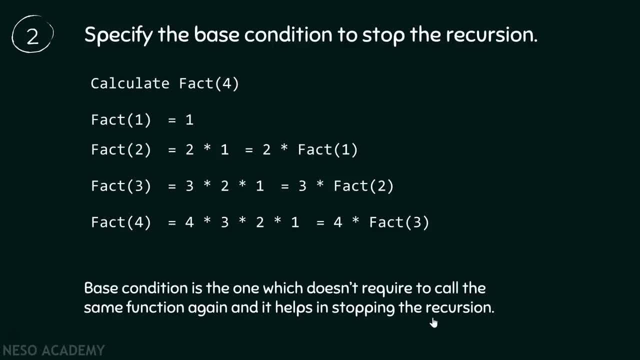 and it helps in stopping the recursion. You should choose the base condition which doesn't require you to call the same function again, Like in this particular case. if you are calculating factorial of three, then you must have to know fact of two. You are calling the same function again, right? 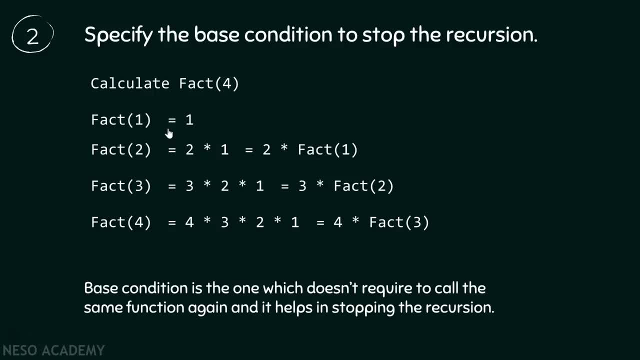 So this cannot be your base condition. But if you observe this line carefully, here you are not calling any function. Fact of one is simply equals to one right. There is no requirement of calling this fact function again, And also it helps in stopping the recursion. 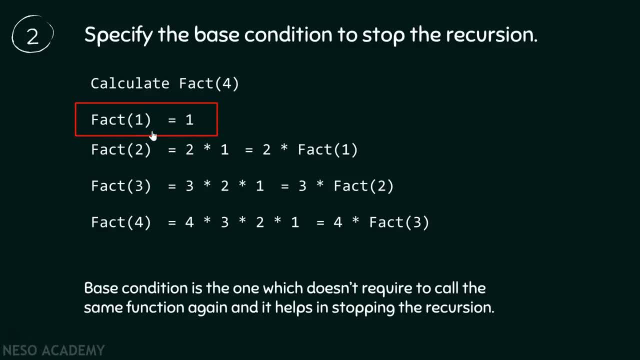 Therefore, I can choose this as my base case, But, remember, you can also choose this as your base case. Here you are simply writing two into one, which is equals to two. finally, right, There is no need to call fact of one. 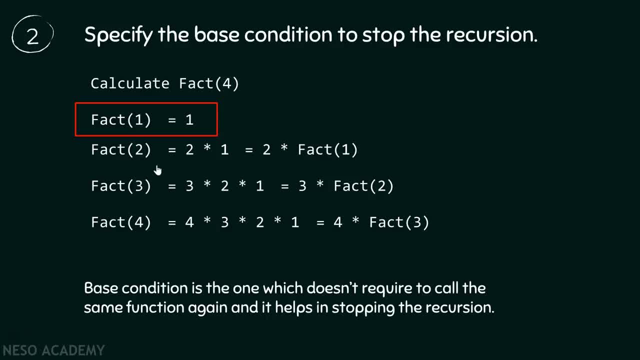 It is just an extra step. You can also write fact of two equals to two and make it as your base case. But for the sake of simplicity we will write this as a base case. If n is equals to one, we simply return one. That's it. 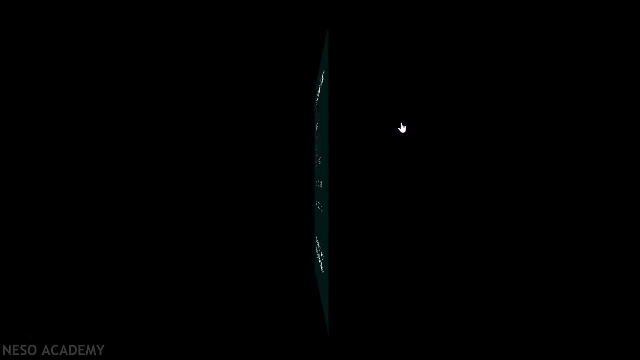 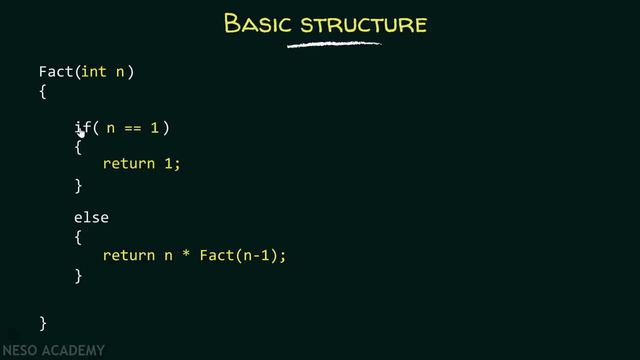 Now let me again get back to the basic structure of factorial function. Here you will simply write your base case as n equals to one and inside this, if construct you mention return one, That's it. This will be your base case. Isn't that simple to write? 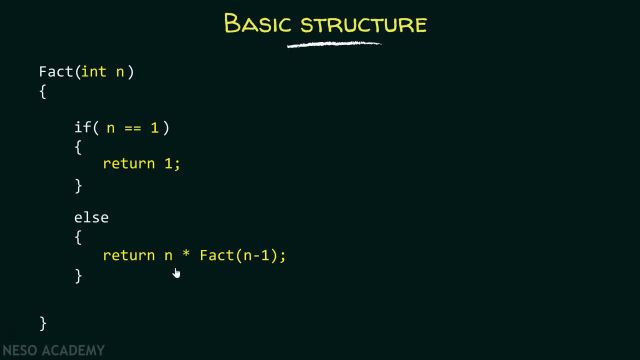 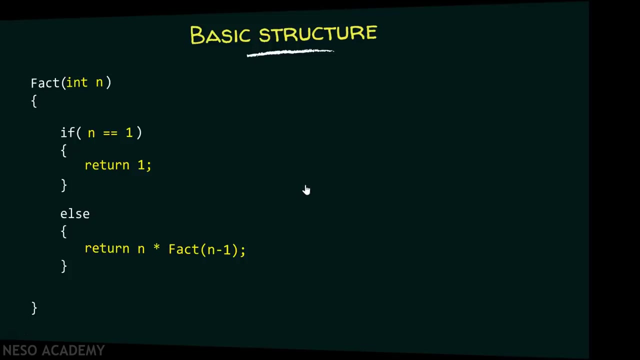 First thing you must have to understand in order to write your recursive procedure is that you have to divide your problem into smaller subproblems So that it will be very easy to decode your problem. After that, specifying the base condition is not that difficult, as you can clearly see, right. 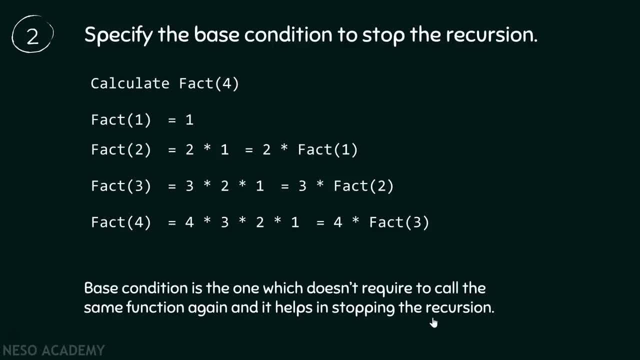 and it helps in stopping the recursion. You should choose the base condition which doesn't require you to call the same function again, Like in this particular case. if you are calculating factorial of three, then you must have to know fact of two. You are calling the same function again, right? 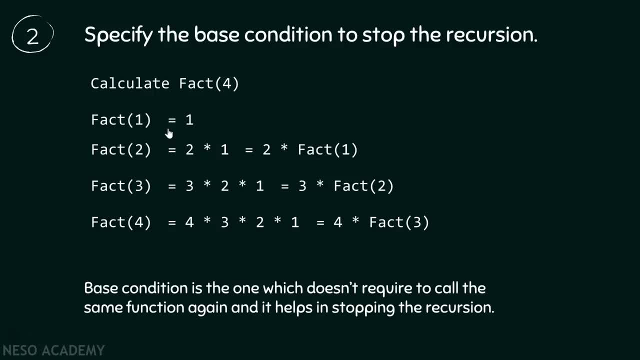 So this cannot be your base condition. But if you observe this line carefully, here you are not calling any function. Fact of one is simply equals to one right. There is no requirement of calling this fact function again, And also it helps in stopping the recursion. 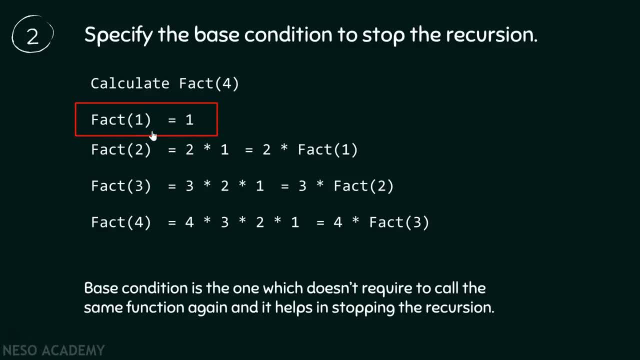 Therefore, I can choose this as my base case, But, remember, you can also choose this as your base case. Here you are simply writing two into one, which is equals to two. finally, right, There is no need to call fact of one. 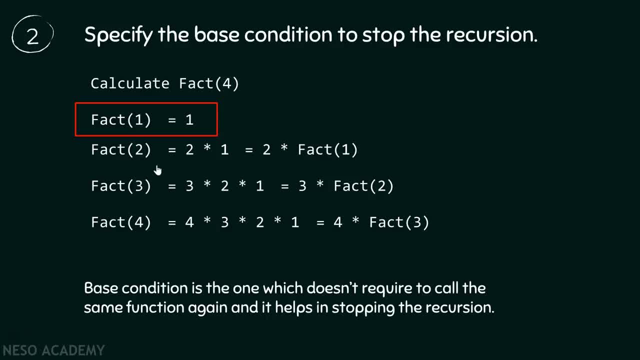 It is just an extra step. You can also write fact of two equals to two and make it as your base case. But for the sake of simplicity we will write this as a base case. If n is equals to one, we simply return one. That's it. 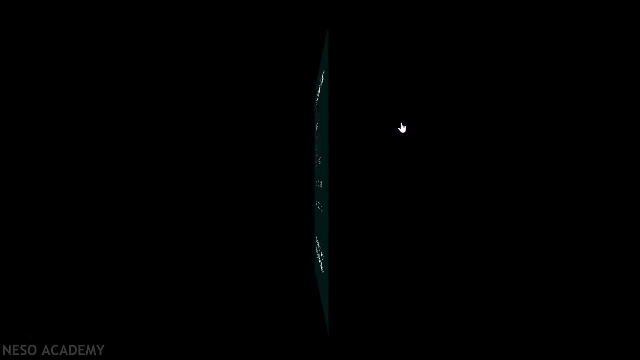 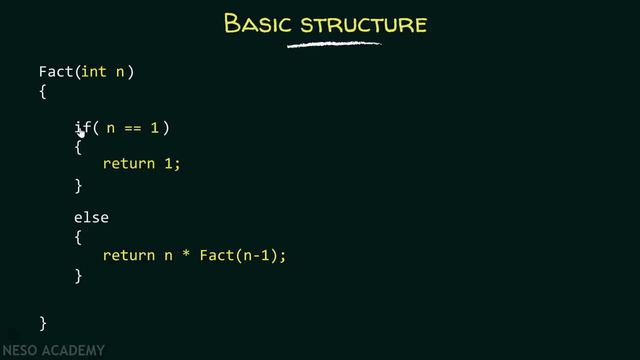 Now let me again get back to the basic structure of factorial function. Here you will simply write your base case as n equals to one and inside this, if construct you mention return one, That's it. This will be your base case. Isn't that simple to write? 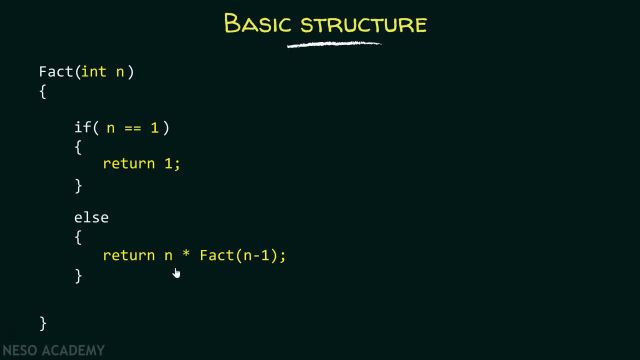 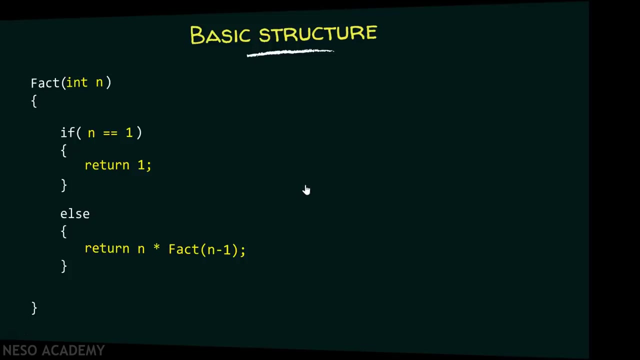 First thing you must have to understand in order to write your recursive procedure is that you have to divide your problem into smaller subproblems So that it will be very easy to decode your problem. After that, specifying the base condition is not that difficult, as you can clearly see, right. 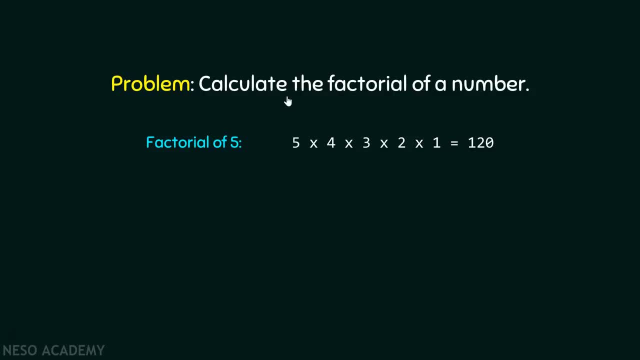 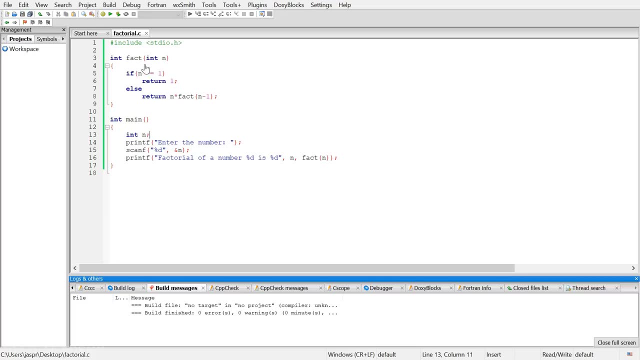 Now, as we know, this is our problem: calculate the factorial of a number. We have already seen the code, Now let's execute the code. Here is the code which helps us in calculating the factorial of a number Inside this matrix: 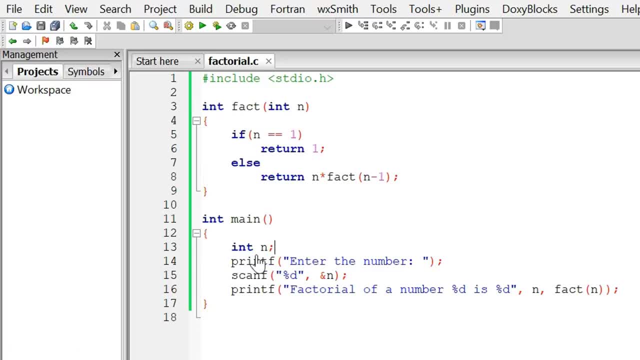 I have declared one variable, n, and then I have written one printf function which says: enter the number. then, with the help of scanf, we are accepting the input from the user. After that, we are printing the factorial of a number by calling this fact of n.